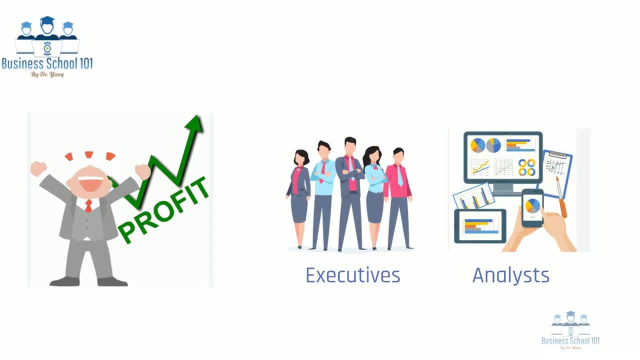 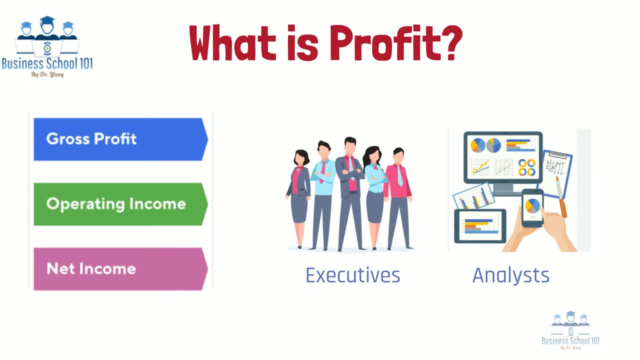 individuals may be required to use basic math to calculate profit on their own. So what is profit? What are the differences between gross profit, operating profit and net income, What is a profit margin and why it is so important? In this video, I will discuss these questions with you. 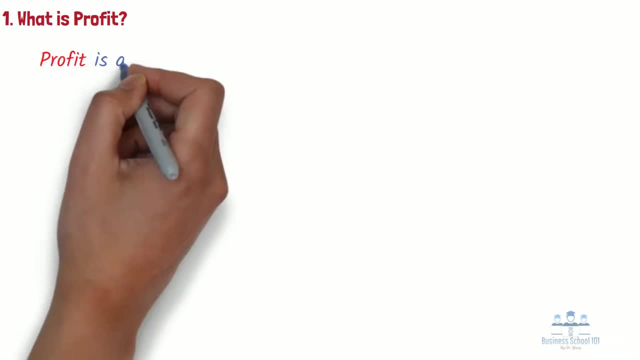 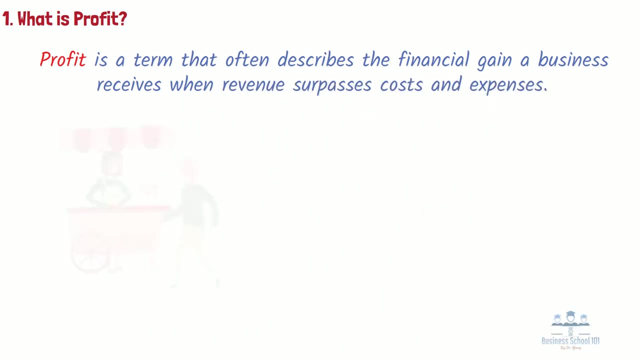 Section 1.. What is profit? Profit is a term that often describes the financial gain a business receives when revenue surpasses costs and expenses. For example, a girl at an ice cream stand spends $1 to create one ice cream cone. She then sells it for $3.. Therefore, her profit on 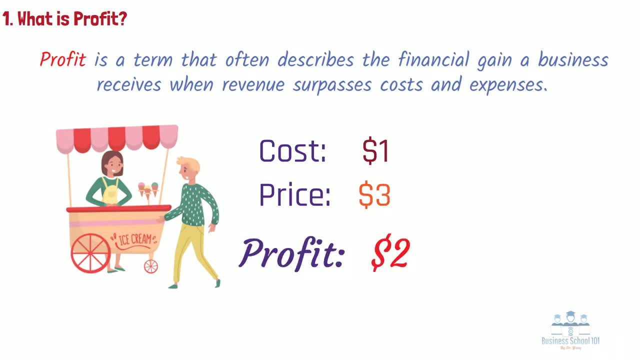 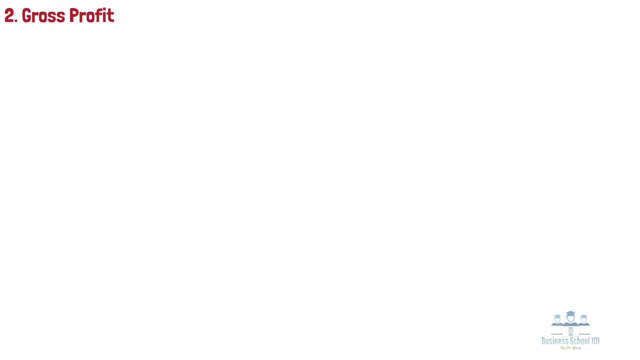 that ice cream cone amounts to $2.. In the real business world, profit can sometimes be a bit more complex, as there are three types of profit: Gross profit, operating profit and net income. Let's discuss them individually: Section 2. Gross profit: Gross profit is the total revenue less only those expenses directly. 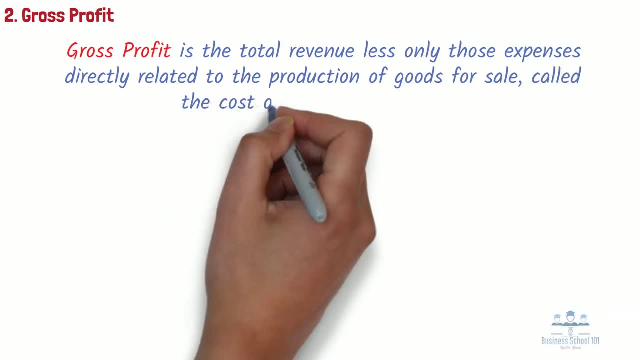 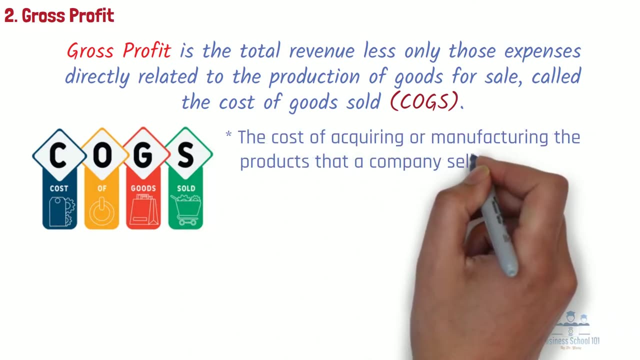 related to the production of goods for sale, called the cost of goods sold or COGS. Please keep in mind that the COGS is the cost of acquiring or manufacturing the products that a company sells in a period, so it only includes costs that are directly tied to the production of the products. 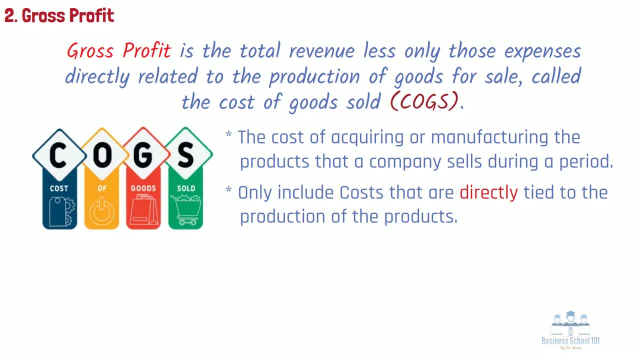 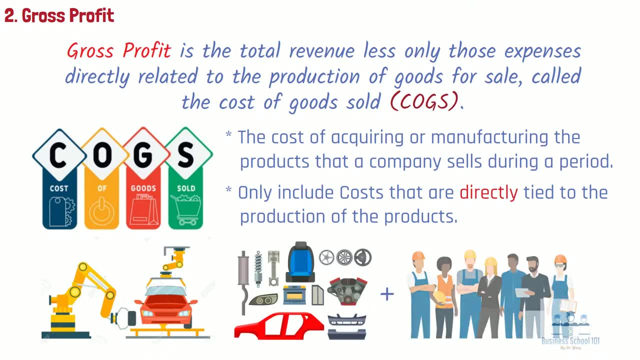 including the cost of labor, materials and manufacturing overhead. For example, COGS for an automaker would include the material costs for the parts that go into making the car, plus the labor costs used to assemble the car. However, the cost of sending the cars to 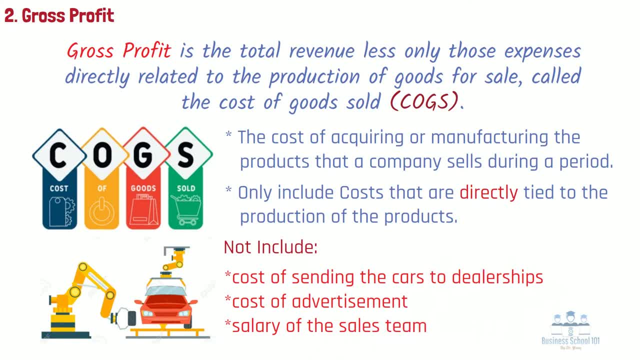 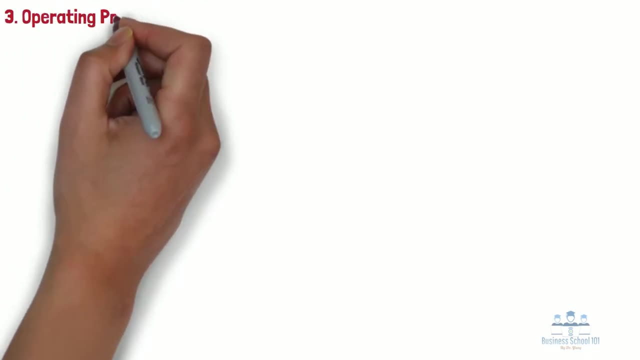 dealerships. the cost of advertisement and the salary of the sales team would be excluded. In addition, gross profit is referred to as gross because it does not deduct debt expenses, taxes or all the other expenses involved in running the company. Section 3. Operating profit Derived from gross profit. operating profit reflects the residual. 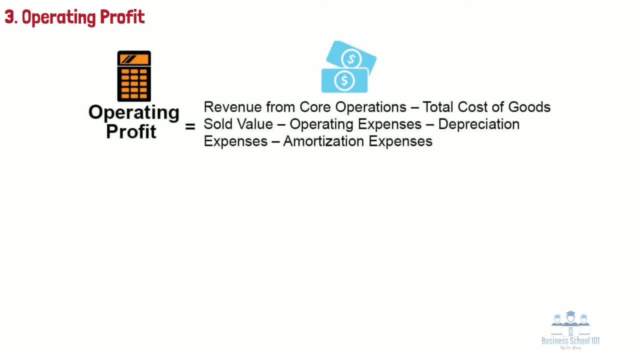 income that remains after accounting for all the costs of doing business. In addition to COGS, operating profit needs to subtract fixed cost expenses such as rent and insurance, variable expenses such as shipping and freight, payroll and utilities, as well as amortization and depreciation of assets- All the expenses 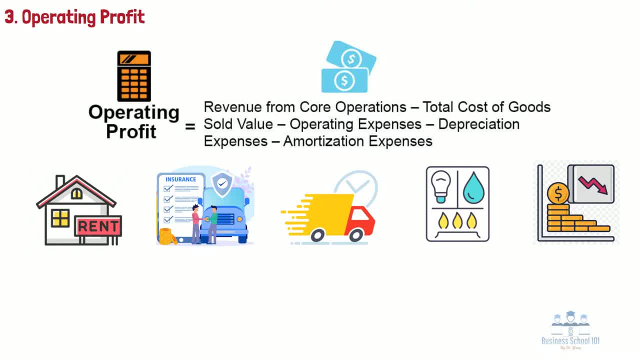 that are necessary to keep the business running must be included. However, like gross profit, operating profit does not account for the cost of interest payments on debts, tax expenses or additional income from investments. Sometimes, operating profit is also referred to as earnings before interest and tax, or EBIT. However, EBIT can include: 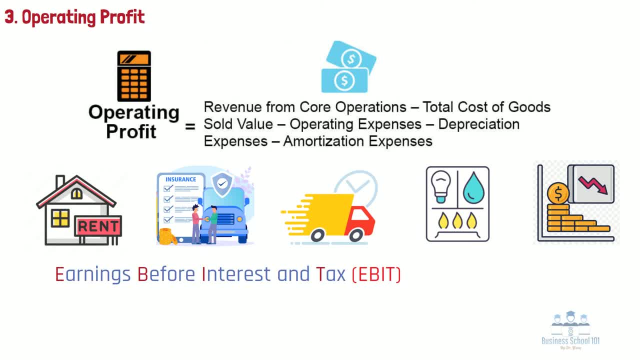 non-operating revenue, which is not included in operating profit. If a company doesn't have non-operating revenue, EBIT and operating profit will be the same figure. In other words, operating profits only reflect the profit and efficiency of a company's core. 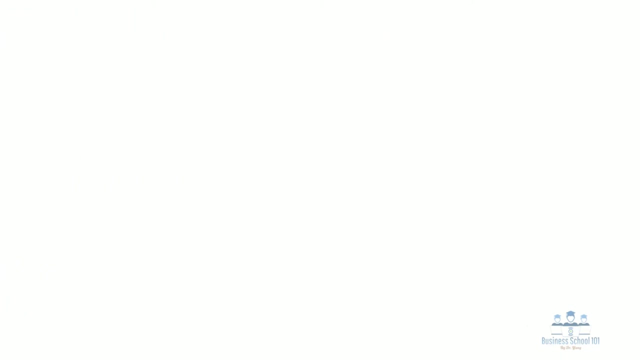 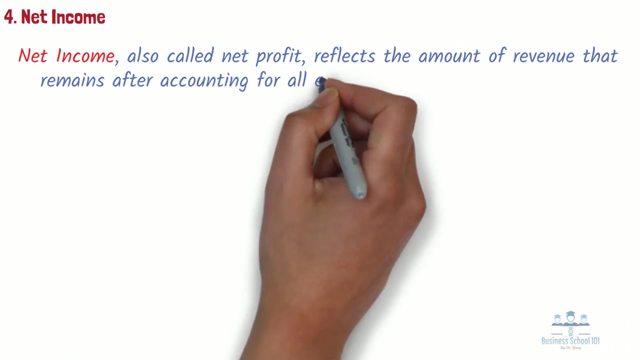 business, Section 4. Net income. Net income, also called net profit, reflects the amount of revenue that remains after accounting for all expenses and income in a period. Net income is the last line and sits at the bottom of the income statement. As a result, it's often referred to. 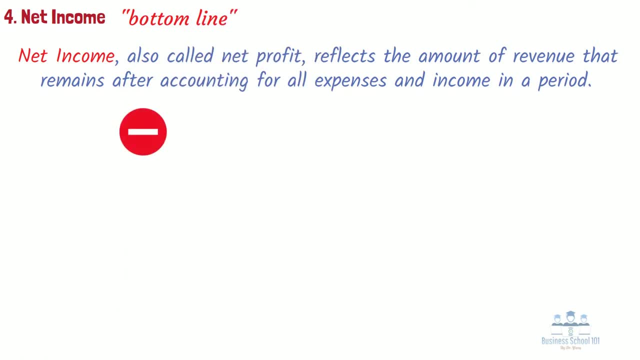 as a company's bottom line number From the operating profit figure. debt expenses such as loan interest, taxes and other expenses are the last line. In other words, net income is the one-time entries for unusual expenses such as lawsuits or equipment purchases are all. 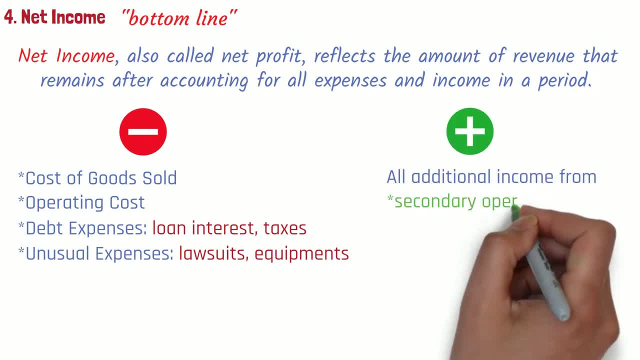 subtracted. All additional income from secondary operations or investments and one-time payments for things such as the sale of assets are added. Net income is arguably the most important financial metric reflecting a company's ability to generate profit for owners and shareholders alike. It's important to note that a company can generate a positive number for operating profit. 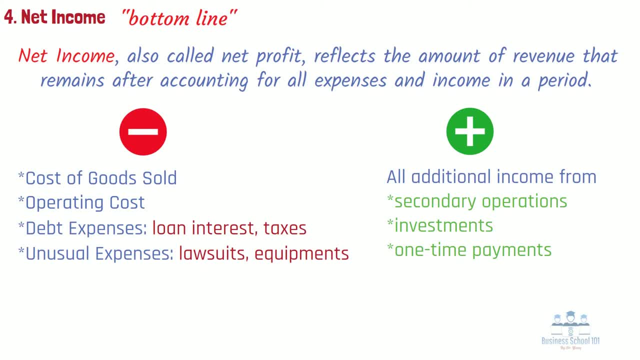 but have a loss or report negative net income. For example, a company generates $100 million in operating profit, but if the interest expense was $110 million for the period, the company would record a $10 million loss in net income despite producing $100 million. 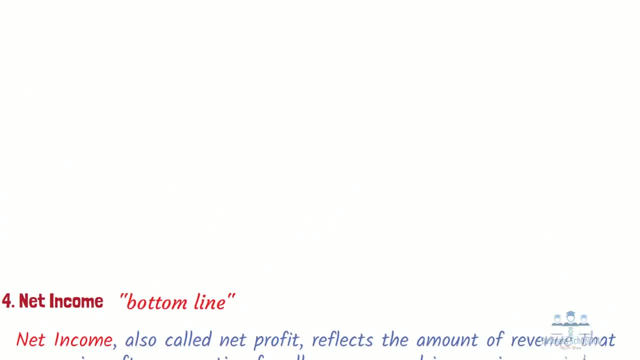 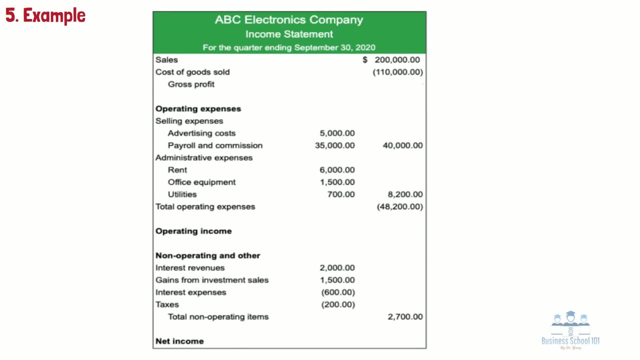 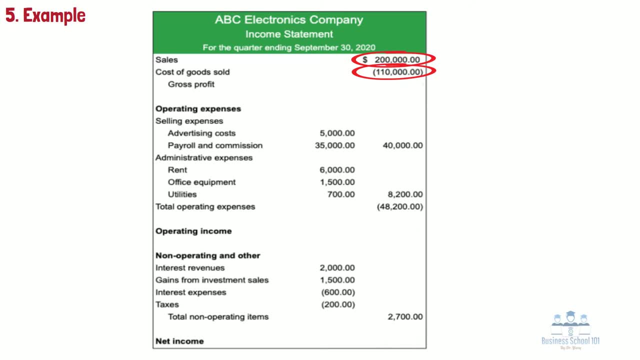 Its gross profit should be sales revenue minus the cost of goods sold: $200,000 minus $110,000, which equals $90,000.. To calculate the operating cost we need to use the gross profit minus all operating costs. In this income statement we can see that ABC Electronics incur five types of 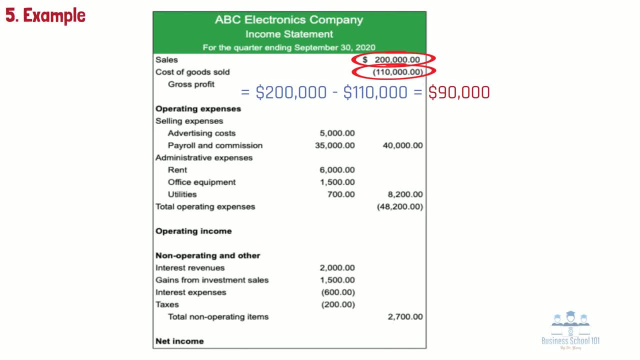 operating expenses, which are advertising, cost $5,000.. Parole and commission cost $35,000.. The rent cost is $6,000.. Office equipment cost $6,000.. Office equipment cost $6,000.. Office equipment. 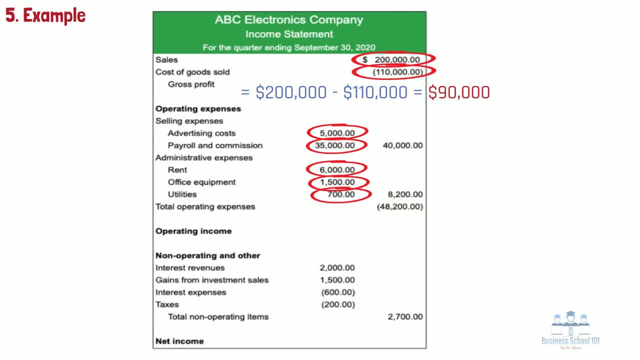 cost $1,500. And the utility cost is $700.. In total, the operating expenses are $5,000 plus $35,000 plus $6,000. plus $1,500 plus $700 equals $48,200.. Therefore, the firm's operating profit should be. 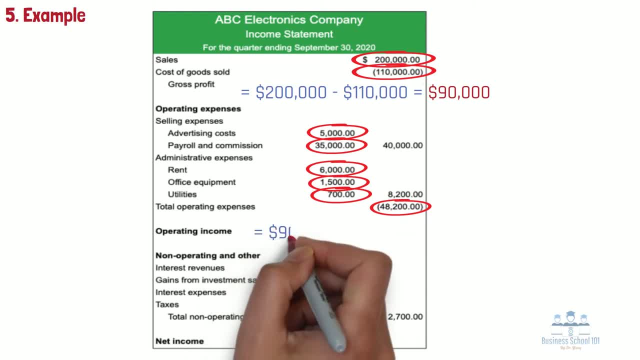 gross profit minus the total operating costs, which is $90,000 minus $48,200 equals $41,800.. Lastly, to calculate the firm's net income, we need to use its operating expenses, which are: $90,000 minus $48,200 equals $41,800.. 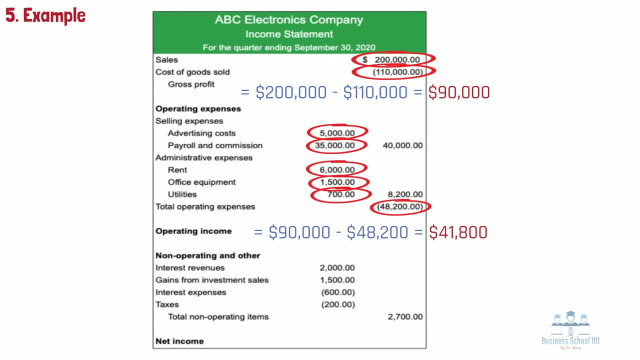 to add the firm's other revenues minus its interest cost and taxes. Within the form you can see the firm has an interest revenue of $2,000.. Gains from investment sales is $1,500.. But it also needs to pay $600 interest and $200 tax. Therefore the firm's total non-operating 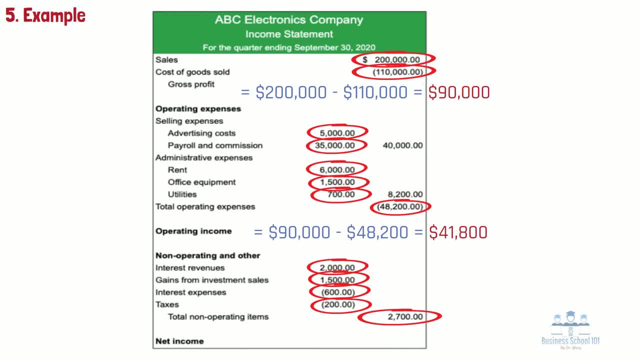 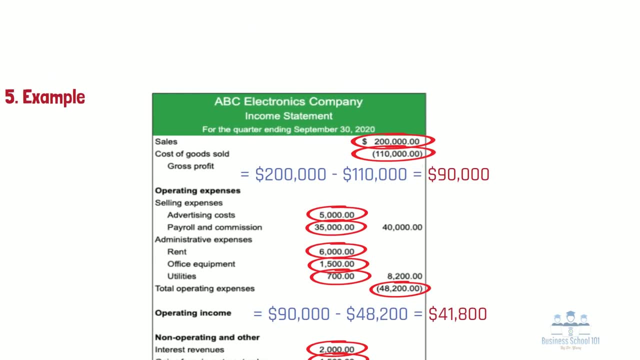 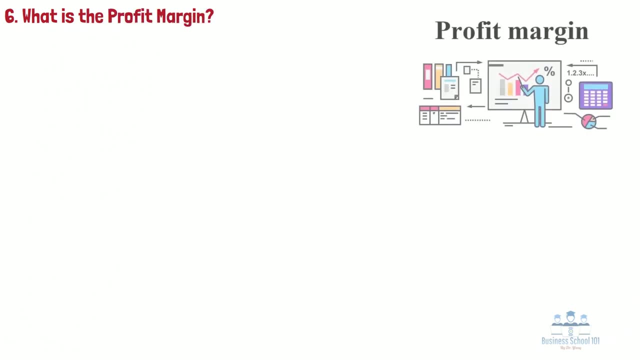 items equals to $2,700, and its net income should be $41,800. plus $2,700 equals $44,500.. Section 6.. What is the profit margin? Profit margin is one of the commonly used profitability ratios to gauge the degree to which a company or a business activity makes money. It represents. 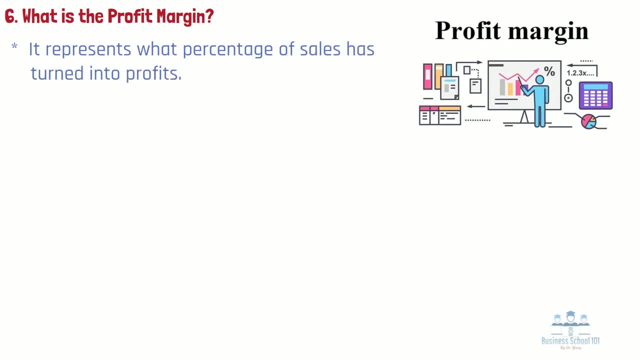 what percentage of sales has turned into profits. Simply put, the percentage figure indicates how many cents of profit the business has generated for each dollar of sale. For instance, if a business reports that it achieved a 35% profit margin during the last quarter, it means that it. 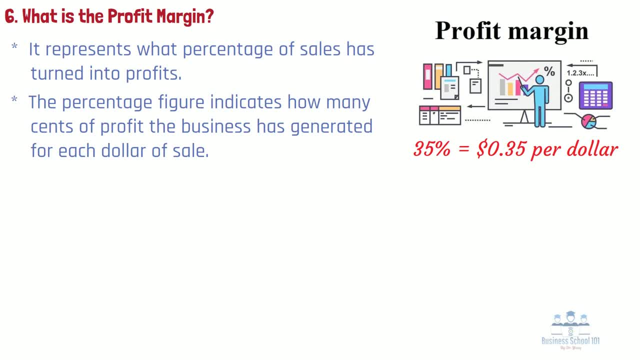 had a net income of $1,000.. For instance, if a business reports that it achieved a 35% profit margin during the last quarter, it means that it had a net income of $1,000.. In accounting and finance there are various ways to calculate the profit margin. Here we only introduce three. 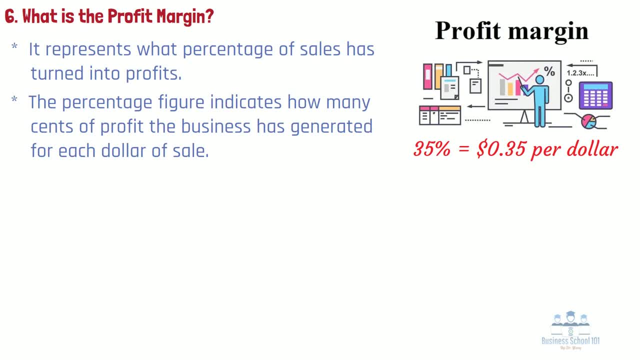 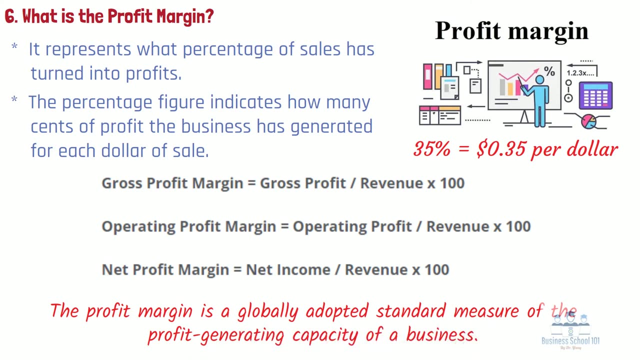 primary margin ratios, which also correspond to three different types of profit: Gross, operating and net. Below is a breakdown of each profit margin formula. The profit margin is a globally adopted standard measure of the profit-generating capacity of a business. Different business participants can use it in various ways. 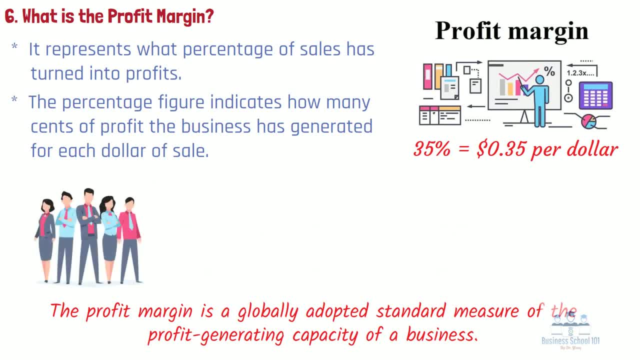 For example: first, business owners, company management and external consultants can analyze profit margins internally for addressing operational issues and to study seasonal patterns and corporate performance during different timeframes. Second, large companies operating multiple business divisions, product lines, stores or geographically spread out. 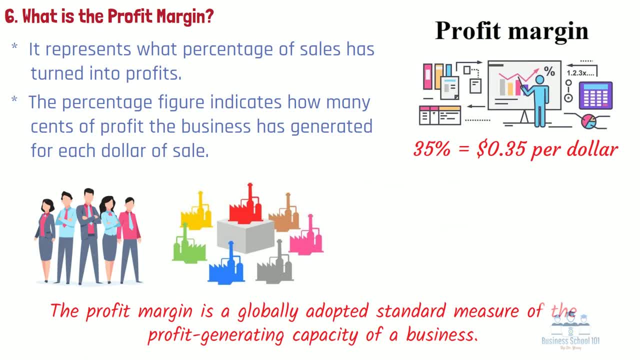 facilities may use profit margins for assessing the performance of each unit and compare it against one another. Third, small companies may use profit margins as proof to seek funding. For example, a local retail store or an auto body shop may need to provide the profit margin for. 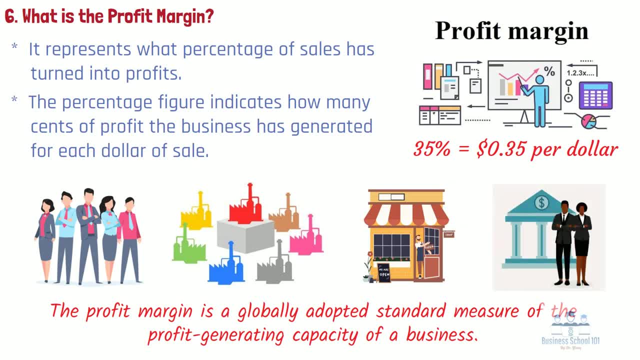 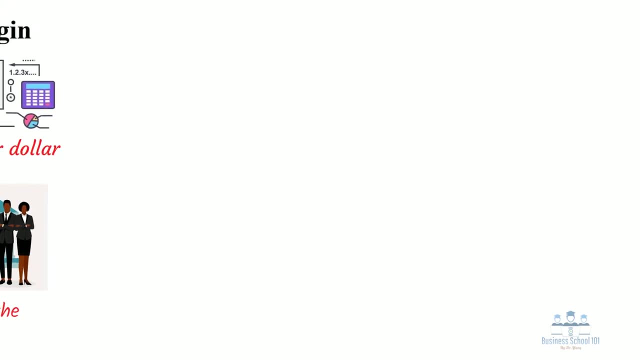 seeking a loan from banks and other lenders. Fourth investors consider the profit margin a critical indicator to evaluate a firm's performance, and potential Investors looking at funding a particular startup may like to assess the profit margin of the potential product or service being developed- Section 7.. 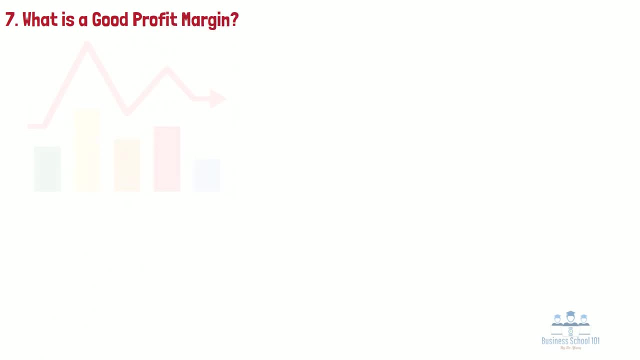 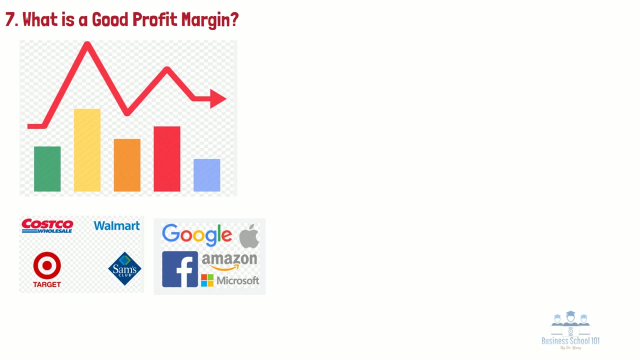 What is a good profit margin? Profit margins vary from industry to industry, which means that companies in different sectors aren't necessarily comparable. For example, a retail company's profit margins shouldn't be compared to those of a technology company. Below is a comparison between the profit margins of four long-running and successful 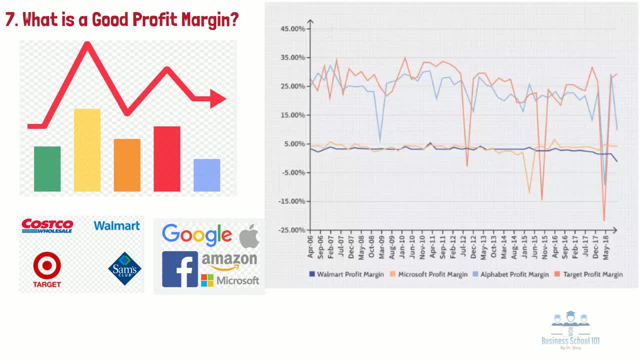 companies in the technology and retail space. As you can see, technology companies like Microsoft and Alphabet have high double-digit quarterly profit margins compared to the single-digit quarterly profit margins. For example, a retail company's profit margins should be compared to the single-digit margins achieved by Walmart and Target. However, 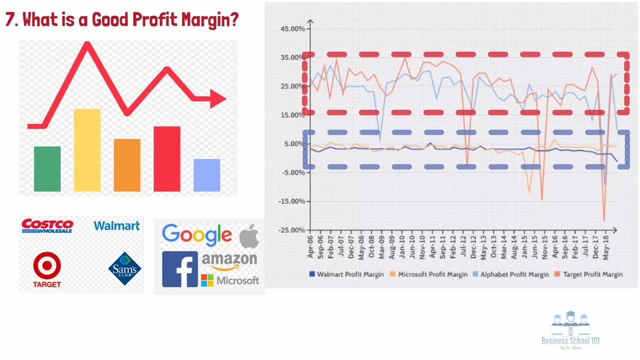 it does not mean Walmart and Target did not generate profits or were less successful businesses compared to Microsoft and Alphabet. To sum up, regardless of what industry the company competes in, business owners need to review their competition as well as their own annual profit margins, to ensure they're on solid ground. 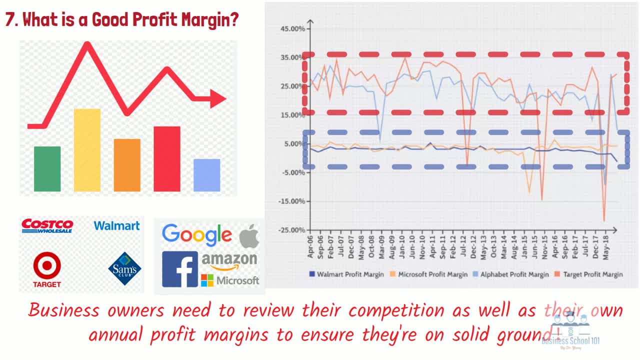 All right, that's all for today's topic. If you have any questions regarding this video, please leave your thoughts in a comment below. I hope that you guys have enjoyed this video And, if you did, make sure you give it a thumbs up and subscribe to my channel. Thanks for. watching and I will see you next time.